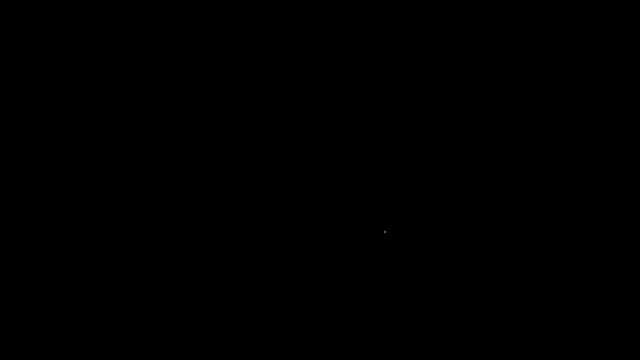 So that's one of the formulas that you need to know. That's the half-angle formula for sine. Now let's do the same with cosine. Let's start with the power reducing formula of cosine squared. So it's 1 plus cosine, 2 theta divided by 2.. So let's divide both angles by 2.. 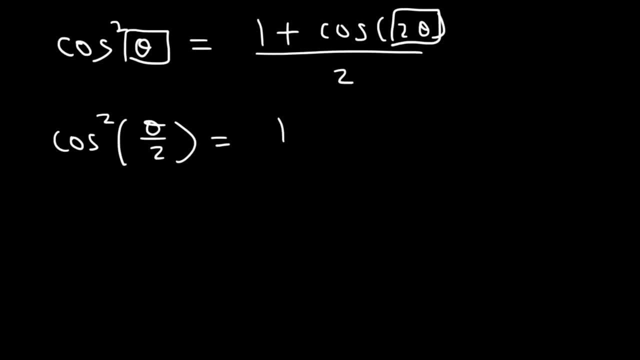 So this becomes cosine theta over 2, and 2 theta will change into theta. Now let's take the square root of both sides. So cosine theta divided by 2 is plus or minus the square root of 1 plus cosine theta divided by 2.. 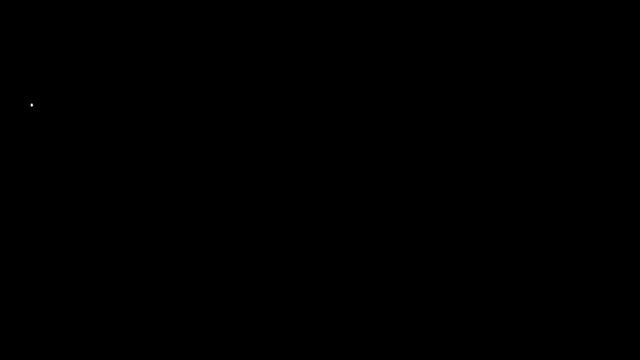 So that's the half-angle of cosines Tangent theta divided by 2 is equal to sine theta over 2 divided by cosine theta over 2.. And sine is plus or minus the square root of 1 minus cosine theta over 2.. 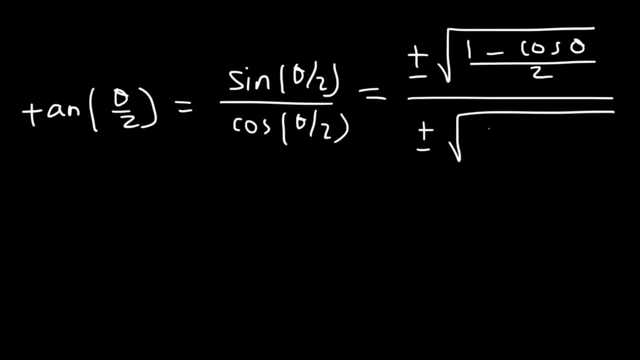 And the formula for cosine is plus or minus the square root of 1 plus cosine, theta over 2.. So we can get rid of the 2s. So what we have now is the square root of 1 minus cosine divided by the square root of 1 plus cosine. 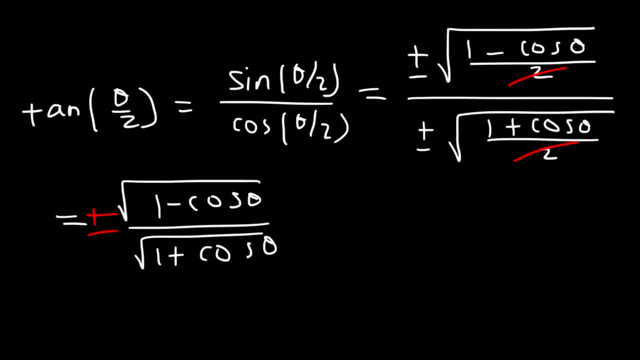 And all we need is a single plus or minus cosine, theta over 2.. So we can get rid of the 2s And all we need is a single plus or minus sine in front. Now let's say if we have the square root of 5 divided by 2.. 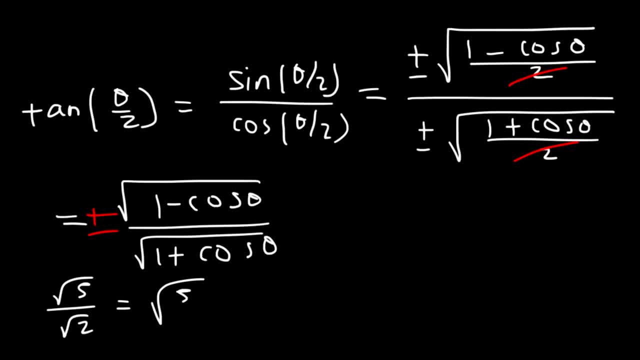 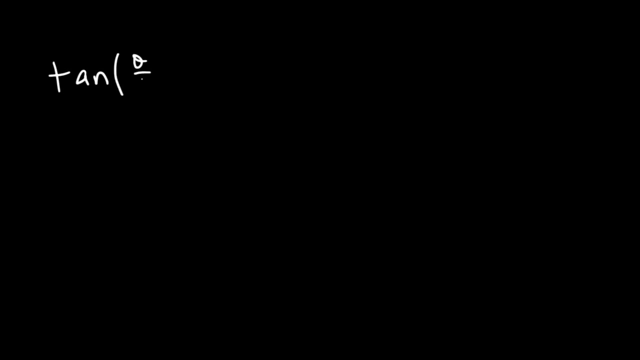 This is the same as the square root of 5 over 2.. So therefore we can say that the half-angle formula for tangent is plus or minus square root 1 minus cosine divided by 1 plus cosine. Now the half-angle for tangent can be calculated using these other two formulas: 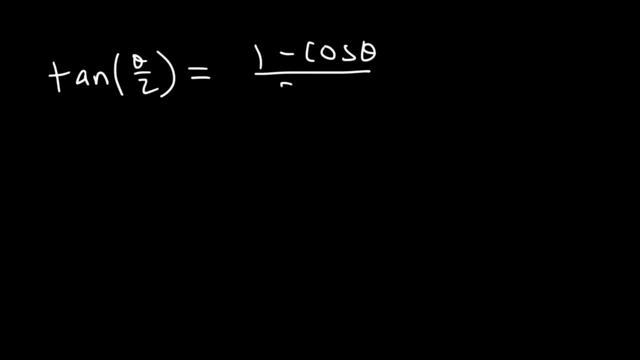 It's also equal to 1 minus cosine divided by sine, And it's equal to sine divided by 1 plus cosine. Use the half-angle formula to evaluate cosine of 15 degrees. Now here's the formula: Cosine- theta divided by 2.. 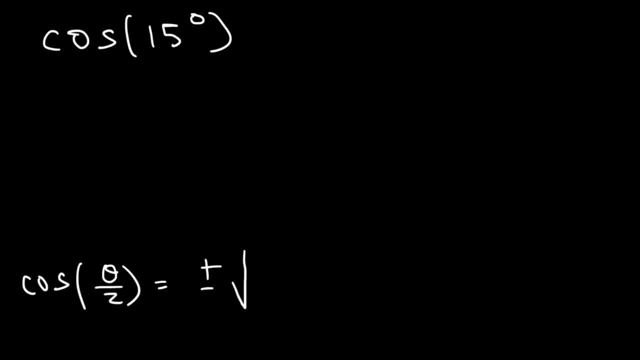 Is equal to plus or minus the square root of 1 plus cosine theta over 2.. So theta divided by 2 is equal to 15.. So if we set 15 equal to theta divided by 2. And if we multiply both sides by 2, we can see that 30 is equal to theta. 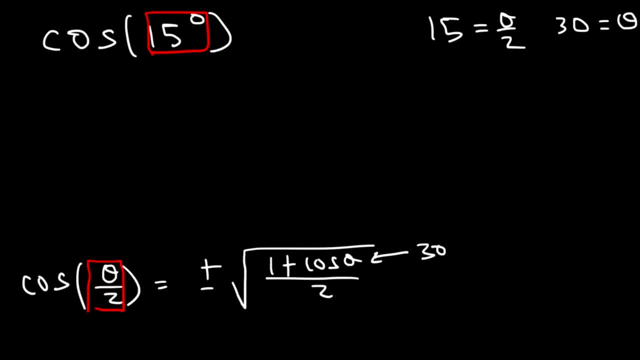 So we need to plug in 30 into this angle here. So cosine 15 is plus or minus the square root Of 1 plus cosine 30 divided by 2.. Now we know the value of cosine 30.. Cosine 30 is equal to the square root of 3 over 2.. 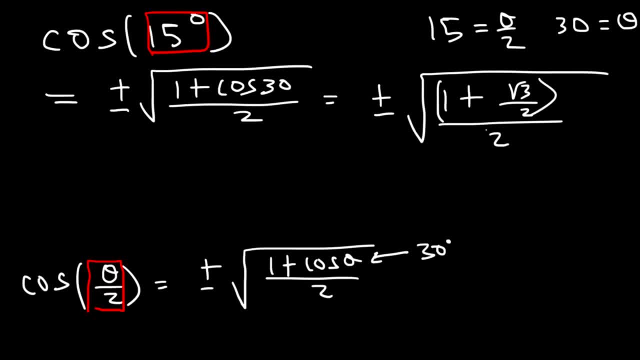 So inside the square root, I'm going to multiply the top and the bottom by 2. To simplify the expression that we have. So first we have 2 times 1., Which is simply 2., And then 2 times the square root of 3 over 2.. 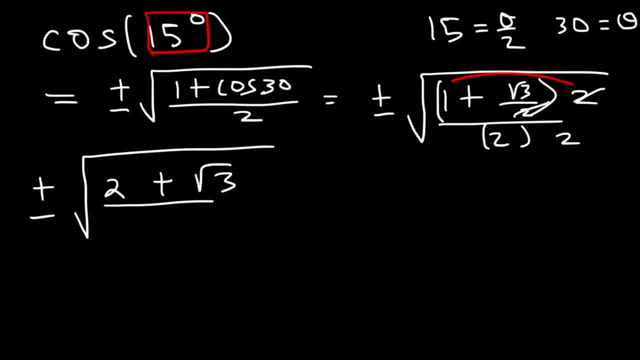 The 2's will cancel And you're just going to get the square root of 3.. And on the bottom we have a 4.. Now the square root of 4 is 2.. So this simplifies to the square root of 2 plus the square root of 3 divided by 2.. 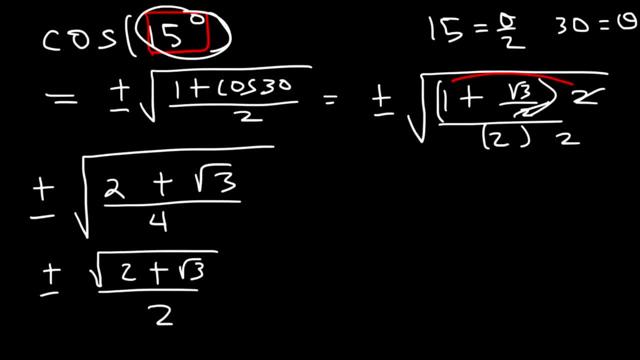 Now 15 degrees is in what quadrant? Quadrant 1,, 2,, 3, or 4.. 15 is an acute angle in quadrant 1.. Cosine is positive in quadrant 1.. So we have 2 signs. 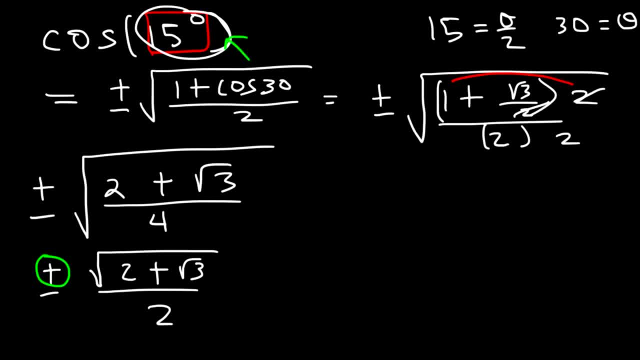 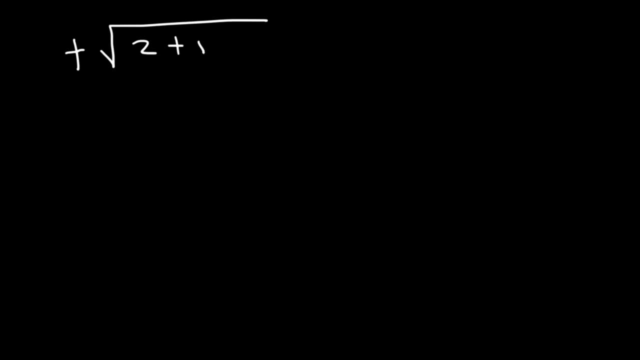 We're going to choose the positive sign based on the quadrant. So the final answer is positive: square root 2 plus square root 3 divided by 2.. Now, if you wish to confirm your answer with a calculator, you can do so. If you get the decimal value of this thing, if you plug it in your calculator. 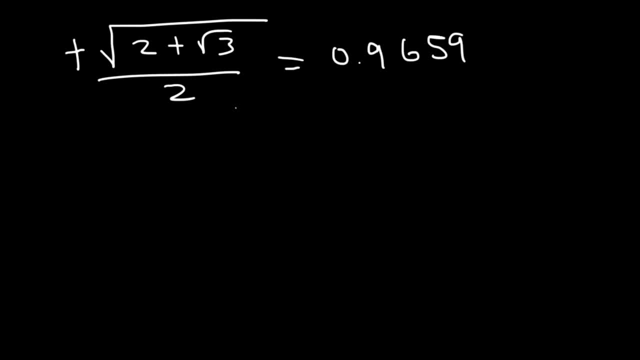 you should get .9659.. Now in some calculators if you type in cosine of 15 degrees, you might get an answer that looks like this: Square root 6 plus square root 2 divided by 4.. It turns out that these two things they have the same decimal value. 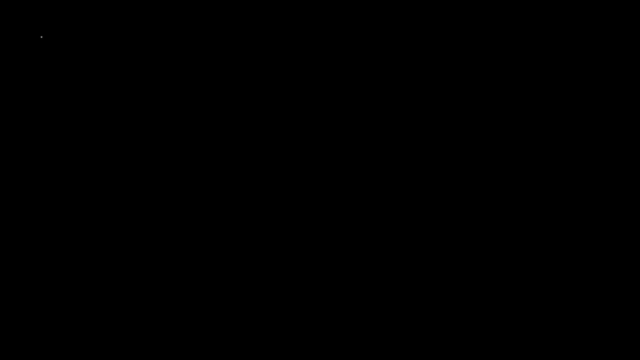 So I just want to point that out. Now let's work on another example. Find the exact value of sine: 22.5 degrees. So feel free to pause the video. Now let's write the formula first. Sine theta divided by 2 is plus or minus the square root of 1, minus cosine theta over 2.. 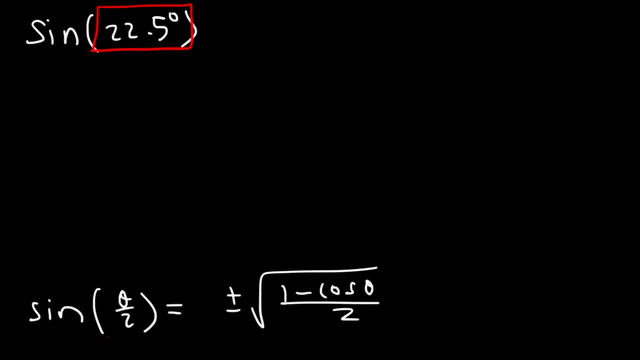 So in this case we can see that 22.5 is equal to theta over 2.. Now, if that's the case, let's multiply both sides by 2.. So the 2's here will cancel, And 22.5 times 2 is 42.5.. 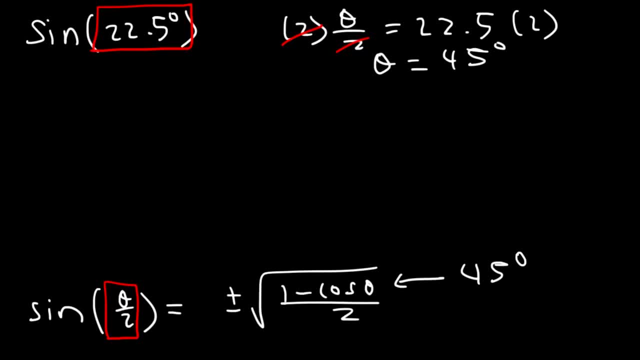 Therefore we've got to plug in an angle of 45 degrees into this expression. So sine of 22.5 degrees is equal. Oh, by the way, is sine going to be positive or negative? 22.5 is in quadrant 1.. 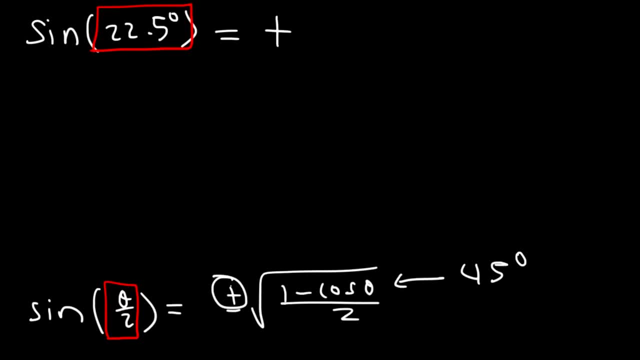 So sine is positive in quadrant 1.. So we're going to use just the positive sine of that equation. So sine 22.5 is positive square root 1 minus cosine 45.. Okay, So sine 22.5 divided by 2.. 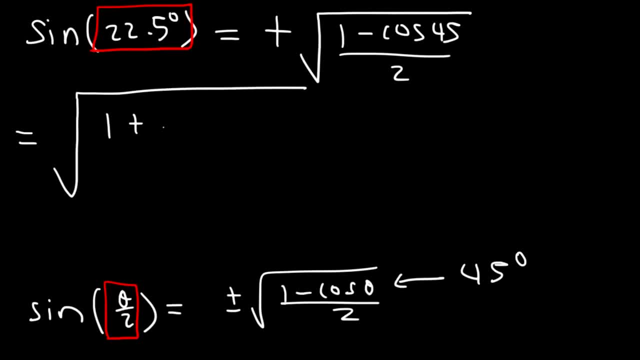 And cosine 45 is square root 2 divided by 2.. So now let's multiply everything, the top and the bottom, by 2 inside the radical. So this is going to be 2 times 1, which is simply 2.. 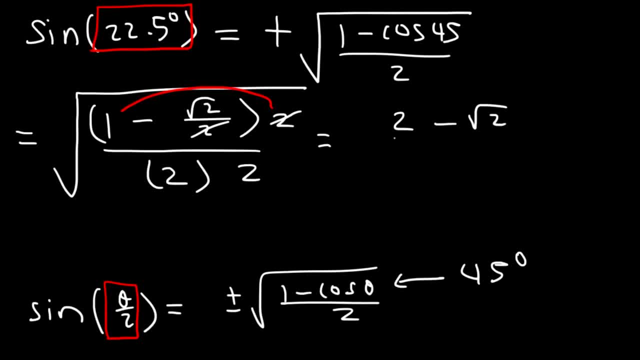 And then these 2's will cancel, leaving behind negative square root 2.. And on the bottom, 2 times 2 is 4.. Now the last thing that we can do is take the square root of 4.. The square root of 4 is 2.. 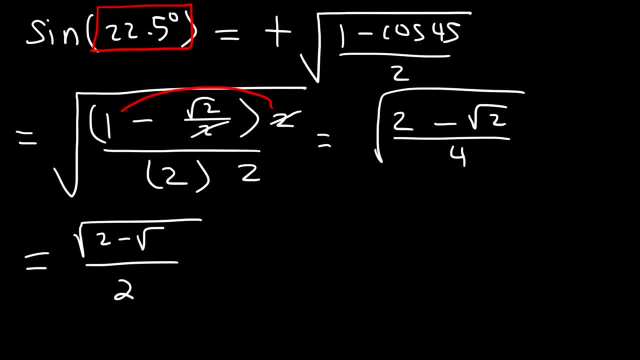 So our final answer is the square root of 2 minus root 2 over 2.. And so that's it. Now let's get the decimal value of that expression. This is equal to 0.3827.. If you type in sine 22.5,, it gives you this value as well. 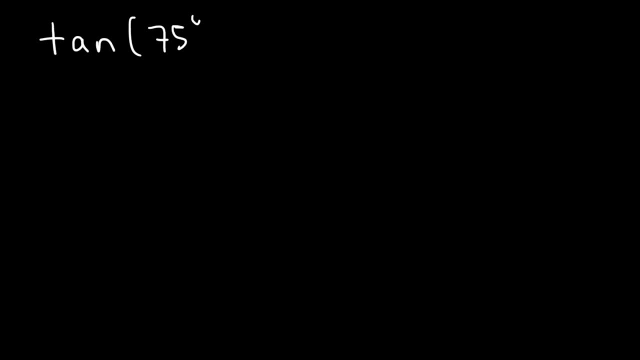 Let's try this one Tangent of 75 degrees. Go ahead and evaluate it. Now I'm going to use this particular formula: Tangent theta divided by 2 is 1 minus cosine theta over sine theta. Now, if theta over 2 is 75,? 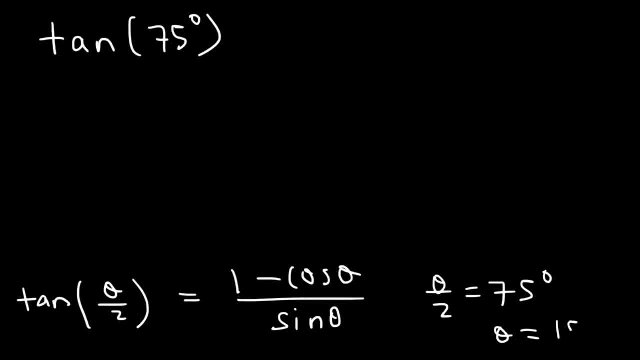 then the angle theta is 75 times 2, or 150.. So tan 75 is 1 minus cosine of 150 degrees, divided by sine of 150 degrees, Now cosine of 150, that has a reference angle of 30.. 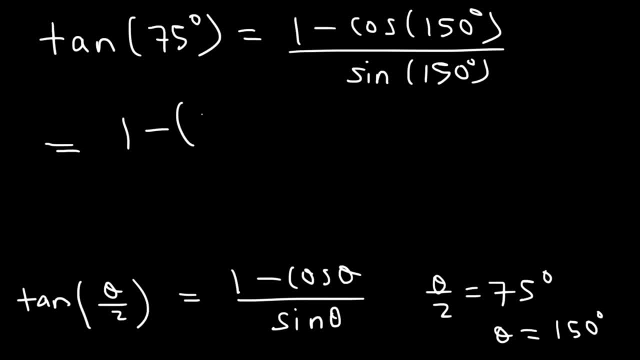 Cosine 30 is the square root of 3 over 2.. But cosine 150, 150 is in quadrant 2, so cosine is negative. So we're going to have negative sine. So we're going to have negative sine. 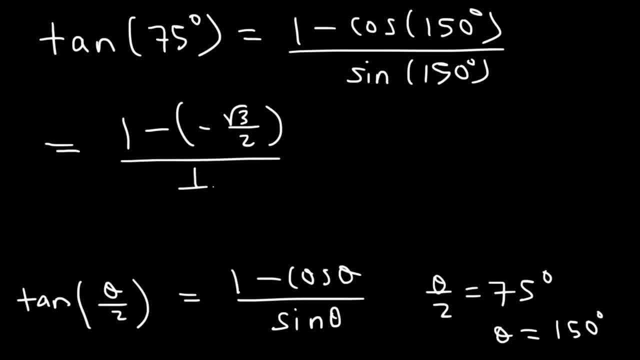 So we're going to have negative sine. So this is the square root of 3 over 2.. Sine 150 is positive 1 half. So this is 1 plus square root of 3 over 2 divided by 1 half. 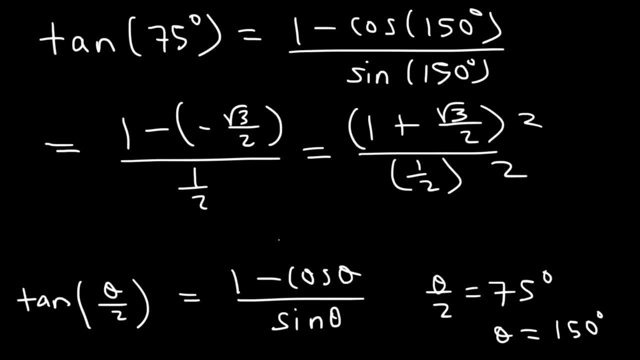 Now let's multiply the top and the bottom by 2.. So let's distribute the 2 on top 2 times 1, that's going to be 2.. And then 2 times the square root of 3 over 2.. 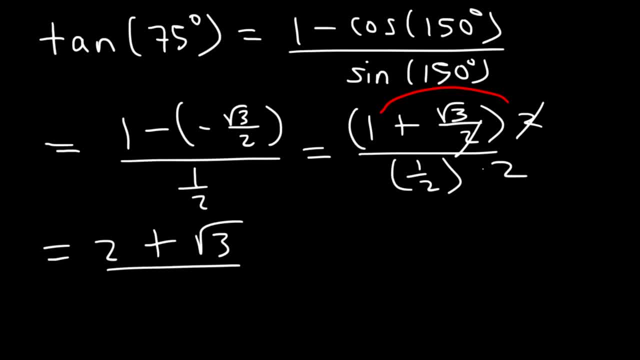 The 2s will cancel, leaving behind the square root of 3.. And 2 times 1 half is 1.. So the final answer is 2 plus the square root of 3. And so that's the value of tangent 75 degrees. 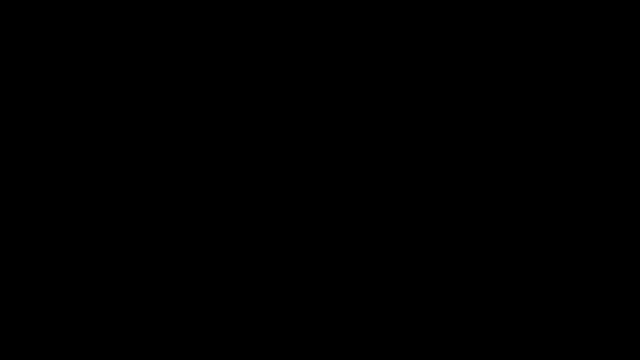 That is the exact value, Thank you.